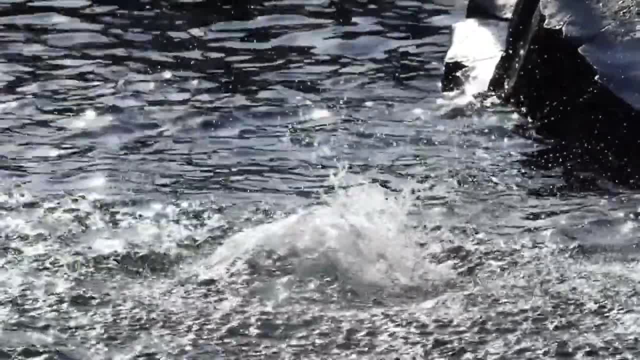 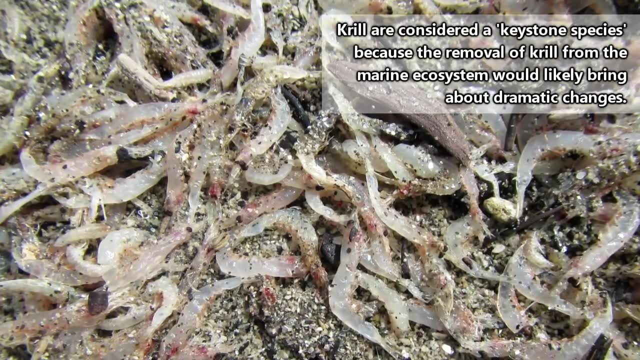 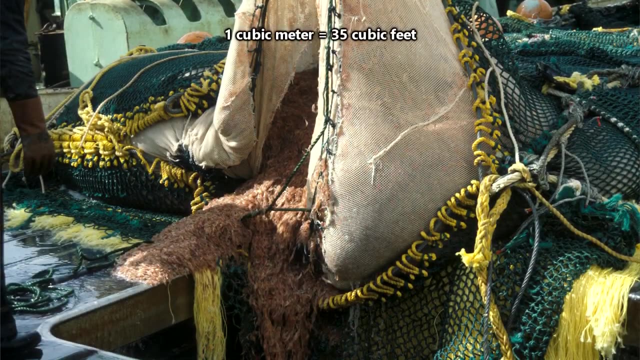 penguins to seals, to fish, to the largest animals living on our planet. the whales depend on krill in order to survive. So, even though they might seem insignificant, krill are one of the foundational aspects of the oceanic food web. Krill are found in groups called swarms In one cubic meter of. 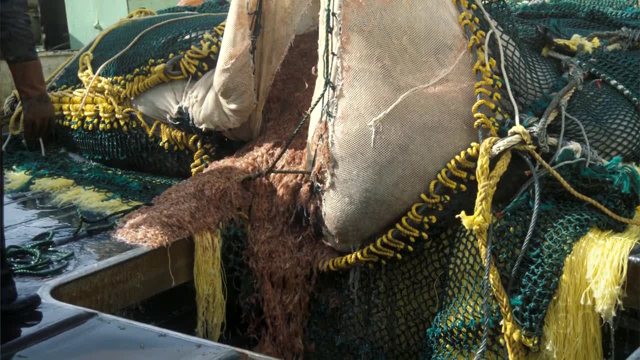 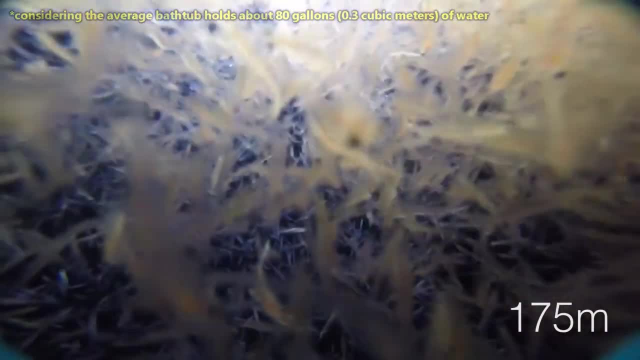 water there can be an average of 10,000 individual krill. To put that into perspective, that would be like having 3,000 individual krill swimming around in your bathtub, And that's just one part of the krill swarm. A swarm of krill may be only a dozen or two feet long, but some swarms. 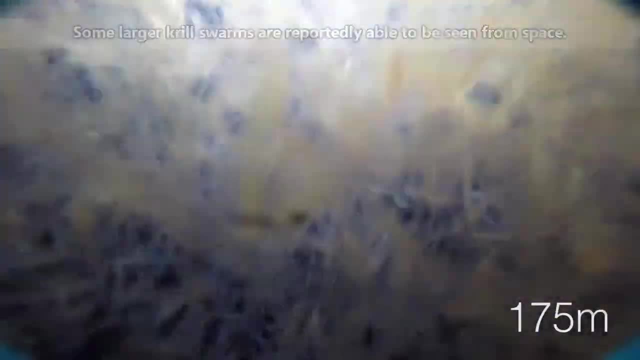 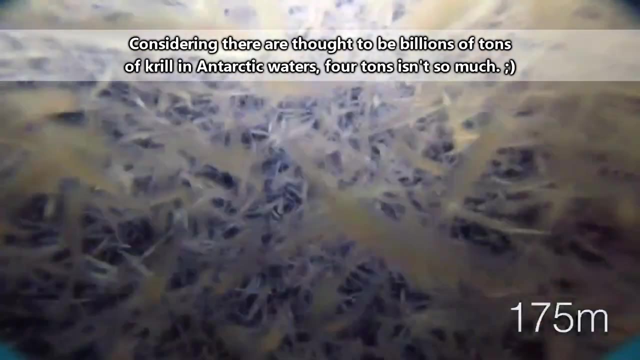 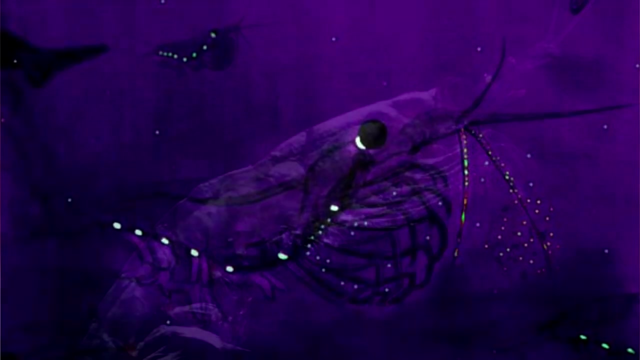 can go on for miles. That amounts to a lot of krill, which is perfect for animals like blue whales, who, during some parts of the year, need to eat four tons of krill per day, And I thought Chester loved food. Being in a group can make finding a mate much easier as well. Some species of krill: 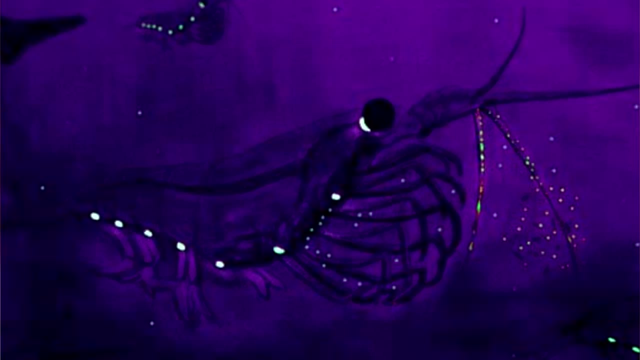 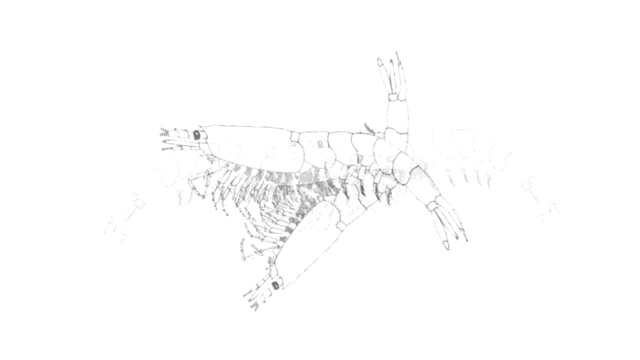 bioluminesce. This may be a means of communication, such as letting all the other krill around know that there's a hungry whale nearby, Or it could also be a means of attracting a mate. Male krill will seek out a female, who he'll basically hug until it's time to part ways. The female will. 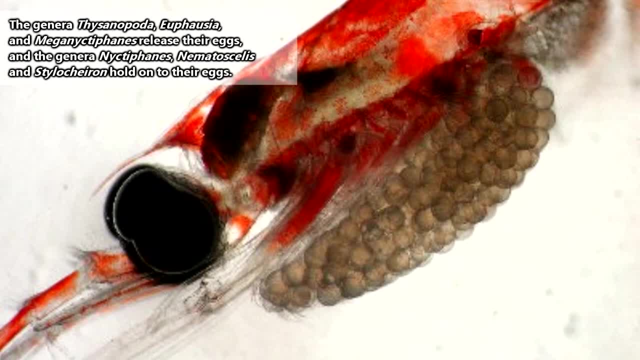 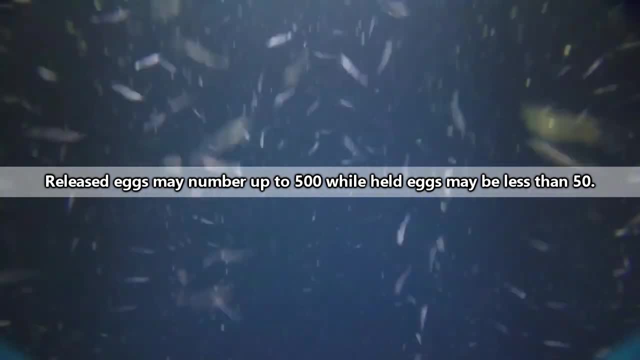 either release her fertilized eggs to sink towards the bottom of the water or they'll hold onto them until they're ready to hatch. Usually, the krill that release their eggs have more eggs at a time, while the ones that hold onto their eggs have fewer Once they hatch krill. 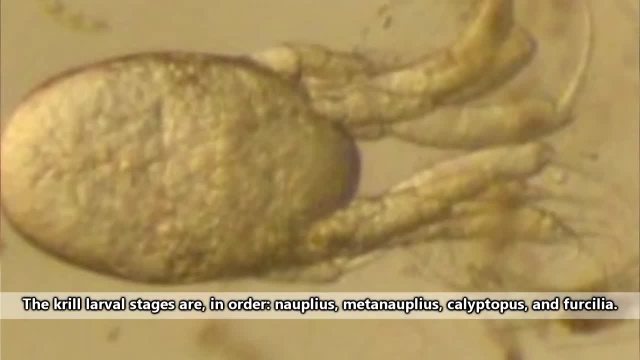 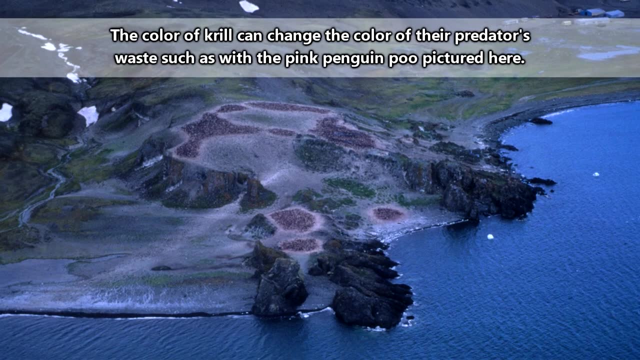 undergo a few life stages, molting as they grow until they reach adulthood. In Antarctic krill specifically, it takes about 10 days for the released eggs to hatch and about 10 days between each larval stage. But this is just one example of how these diverse creatures develop. Some species. 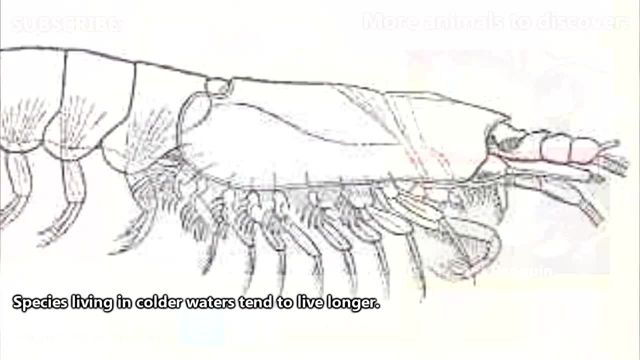 may live less than a year, while others can live up to a year. Some species may live less than a year, while others can live up to a year. Some species may live less than a year, while others can live to be 5 or older. For more facts on krill, check out the links in the description. Give a thumbs. 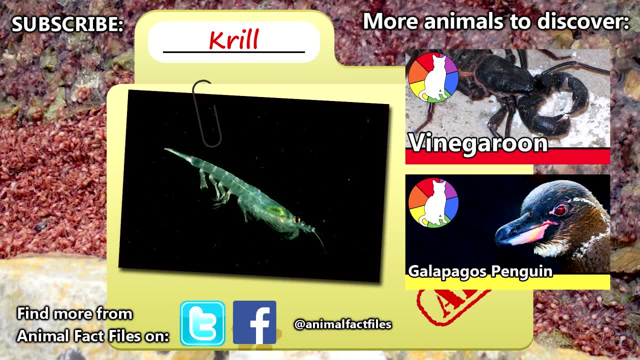 up if you learned something new today and thank you for watching Animal Fact Files.